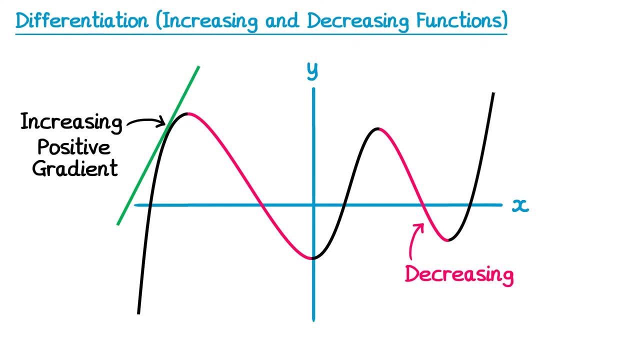 therefore it has a positive gradient. If it has a positive gradient, then the gradient function dy by dx must be positive as well, so it must be greater than zero In the red section. however, if we draw a tangent, it will be sloping downwards. 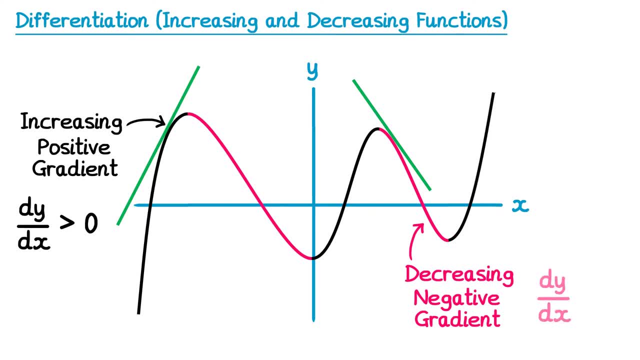 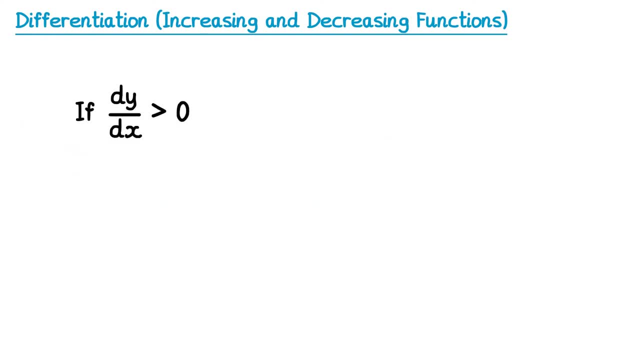 So it has a negative gradient, in which case, dy by dx, the gradient function, must be less than zero. This leads us to be able to make two statements about functions. If dy by dx is positive, the function is increasing. If dy by dx is negative, then the function is decreasing. 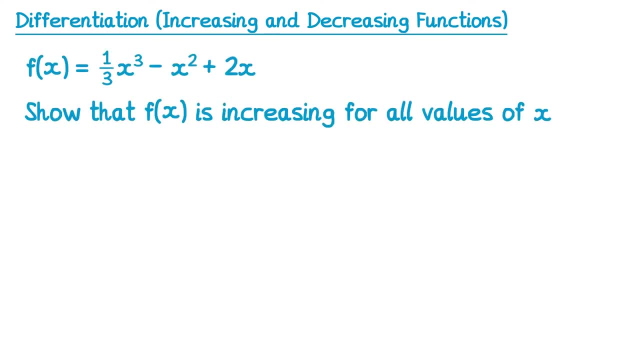 Let's have a look at how we can apply this to questions. Here. we have a function and we're asked to show that it is increasing for all values of x. If it is increasing, then dy by dx must be greater than zero. 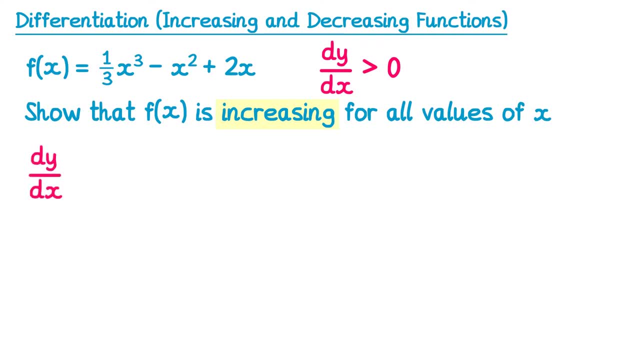 So let's work that out. So, dy by dx, we do 3 times the third, which is just 1, and then reduce the power of x cubed down to x squared, so it's just x squared. If we differentiate negative x squared, we get negative 2x, and if we differentiate plus, 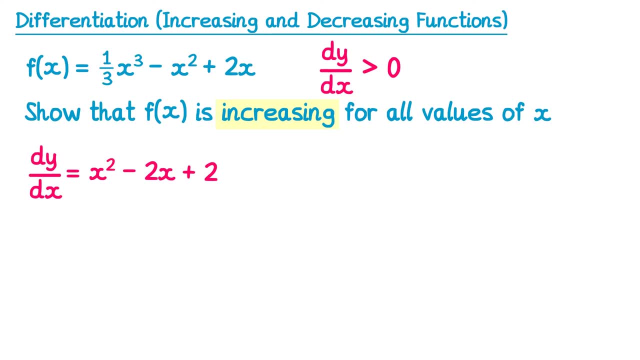 2x, we get plus 2.. So we've found dy by dx, and we need to show that this is always positive. To show something is always positive, or indeed always negative, the easiest way is to complete the square. So we'll complete the square on this. so this is equal to a bracket squared. 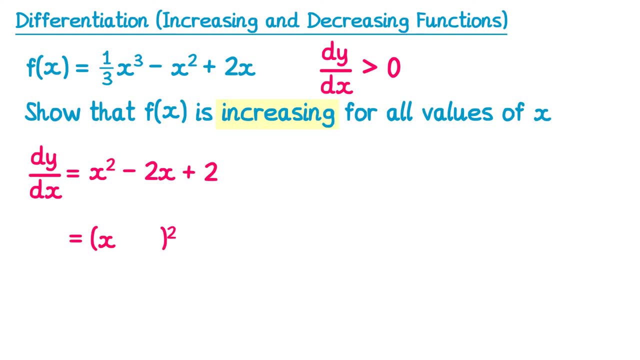 Inside the bracket we need to halve the coefficient of x. at the moment it's negative 2, so we'll stick a negative 1 in here. We then square that negative 1, which gets you 1, but then subtract it, so subtract 1,. 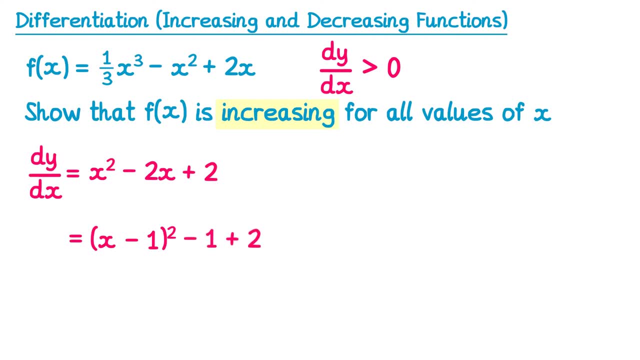 and then bring this plus 2 down and the negative 1 plus 2 will give you plus 1.. Now it's in this form we can actually show that it is always positive. This first bit here is just the bracket squared. 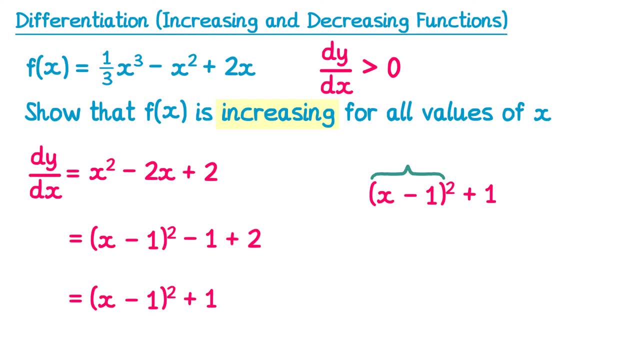 So whatever number of x we substitute in here, this must be greater than or equal to 0, since square numbers can't be negative, Even if x was a negative number, for example negative 5,, we'd get negative 5. take away: 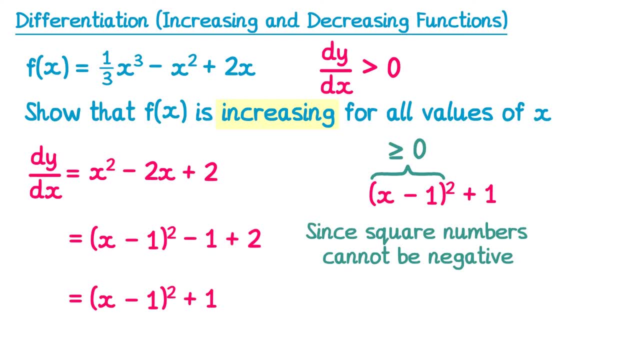 1,, which is negative 6, and then you square that and it becomes positive. So this can't be less than 0.. So the lowest value this bracket squared could be is 0, and then we're going to add 1 to. 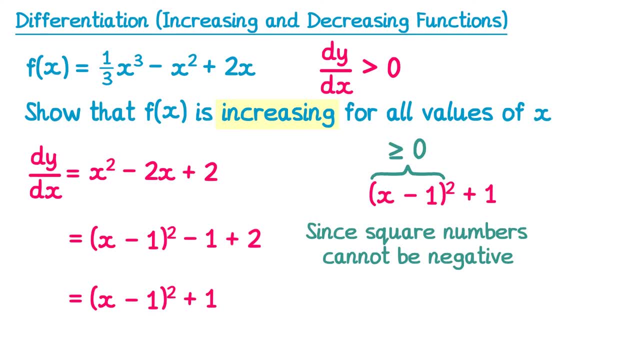 that. so the lowest value dy by dx could be is 1.. So dy by dx is greater than or equal to 1.. So dy by dx is greater than or equal to 1.. And 1,, of course, is greater than 0,, in which case f of x is increasing. 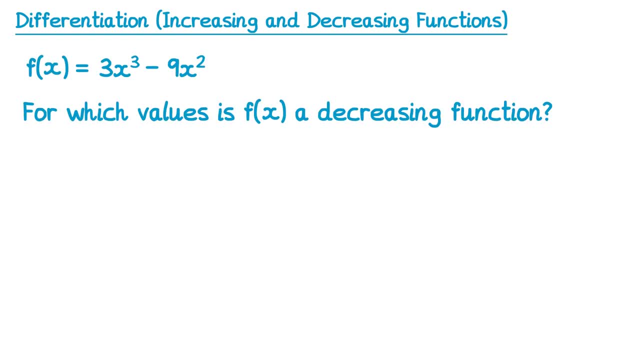 For this question. we have another function and we're asked to find the values for which f of x is a decreasing function. If f of x is decreasing, then we know that dy by dx is less than 0. So let's work out dy by dx. 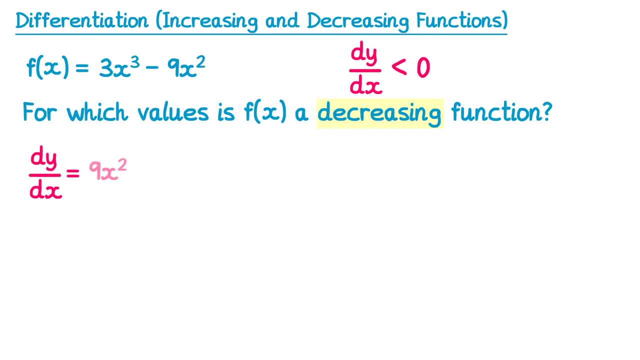 3 times 3 is 9, and reduce the power from x cubed to x squared, so 9x squared, and then do 2 times negative 9.. So negative 18, and reduce the power from x squared to just x, so negative 18x. 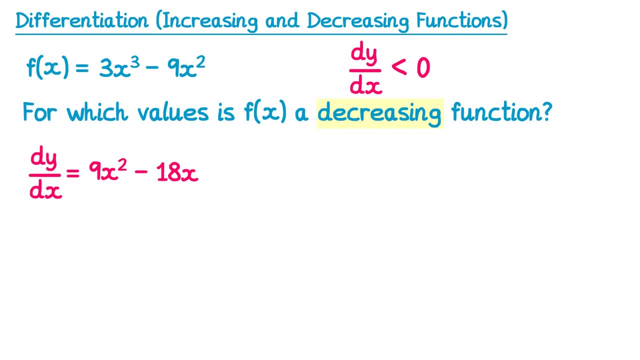 Now this time we need to actually find the x values for which it is decreasing. So we want the gradient function to be less than 0, so let's write: 9x squared minus 18x is less than 0.. Now we end up with a quadratic inequality that we need to solve. 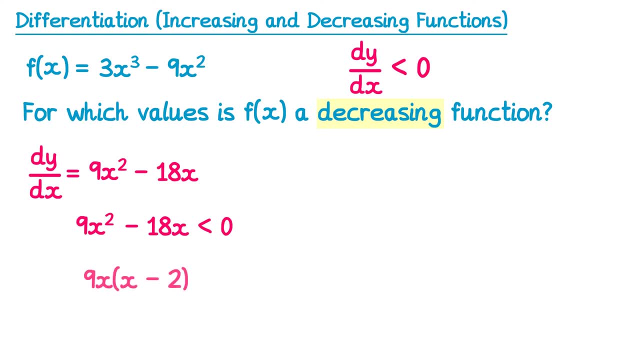 We can factorise the left hand side. If you factorise 9x out, you get 9x, and then x take away 2, which is less than 0. This gives us two critical values. The 9x will give us a critical value of x equals 0, and the x take away 2 gives a critical. 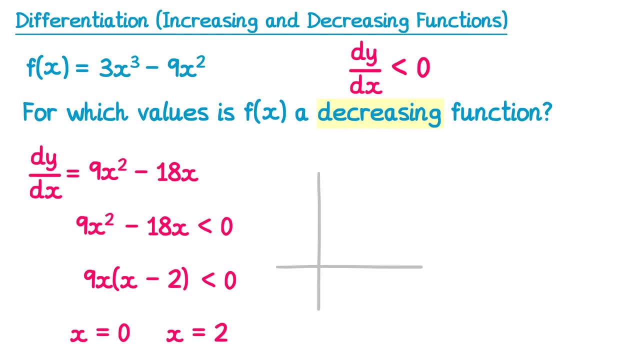 value of x equals 2.. So if we drew the graph of this, it would cross at 0, and 2, and it's a quadratic, so we'll get that classic u shape. We want to know when this graph gives a value less than 0.. 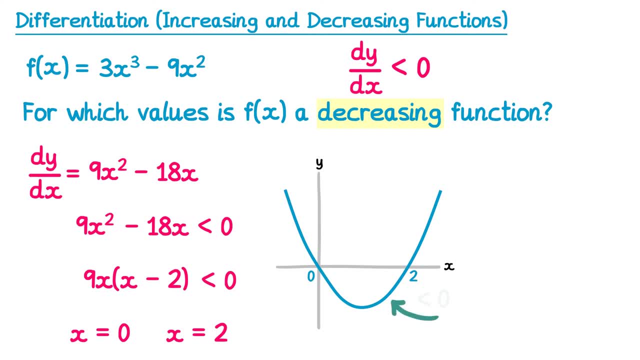 This corresponds to the section where we're below the x axis, since that's less than 0. The x values that keep us below the axis are in between 0 and 2.. We've found the solution to this inequality. It's: x is in between 0 and 2.. 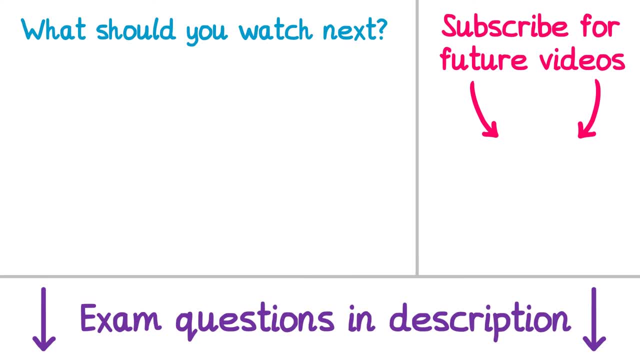 Thank you for watching this video. I hope you found it useful. Remember there are some exam questions in the video's description. Check the video. I think you should watch next and subscribe so you don't miss out on future videos.